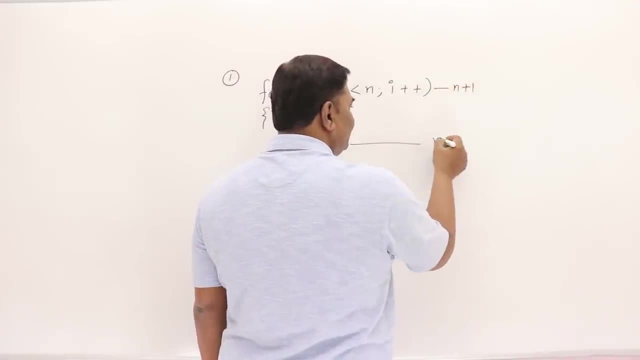 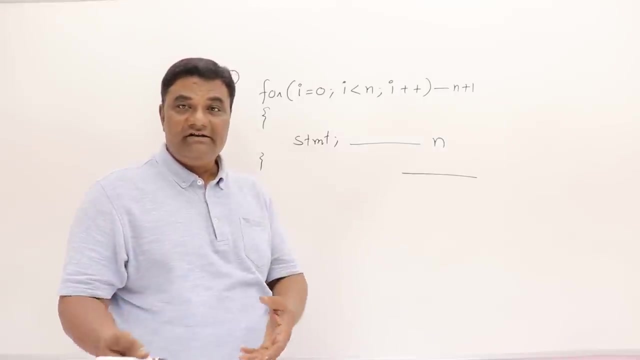 We know that this will execute for n plus one time and this will execute for n time. We don't want this time because, anyway, when we are writing order of, we are writing a degree, So this will not affect the degree at all, So it will be same, only So. just we need to know the 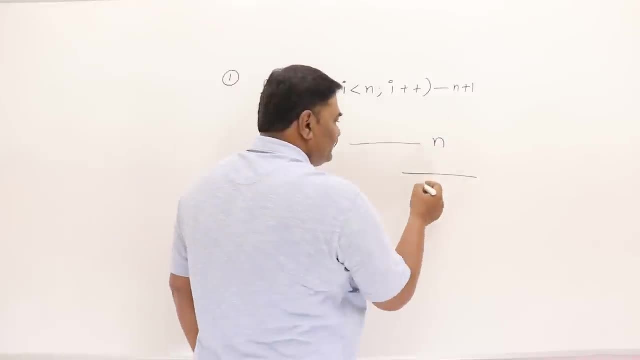 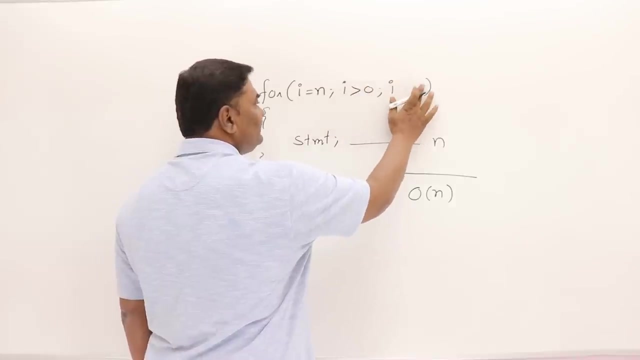 statement how many times it is executing. So that's it. So this is order of n. You can avoid this one. Skip this one. Next, if suppose this loop is starting from n and the condition is greater than 1 or 0, and this: 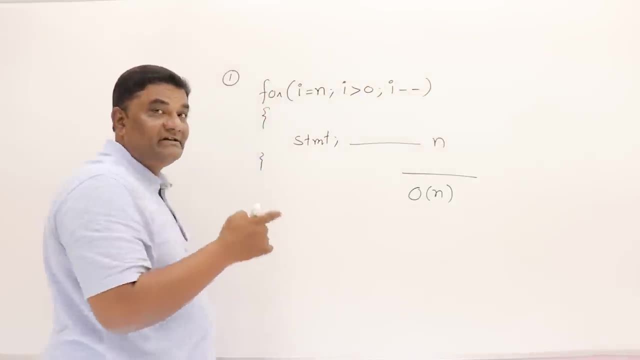 is getting subtracted, So this loop is decrementing. Then also this statement will execute for n times and it's order of n. Whether you go from 1 to 10, 10 steps, or come from 10 to 1, then also 10 steps. So you go from 1 to 10 or 10 to 1.. Same. 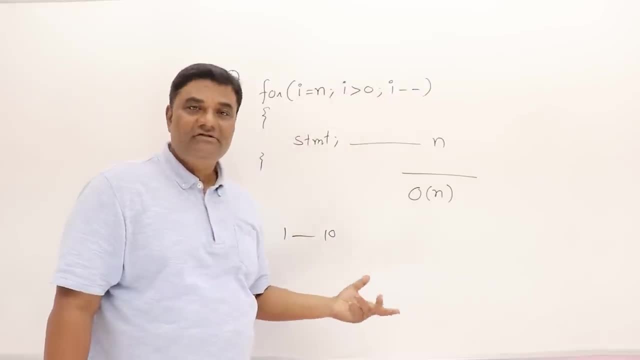 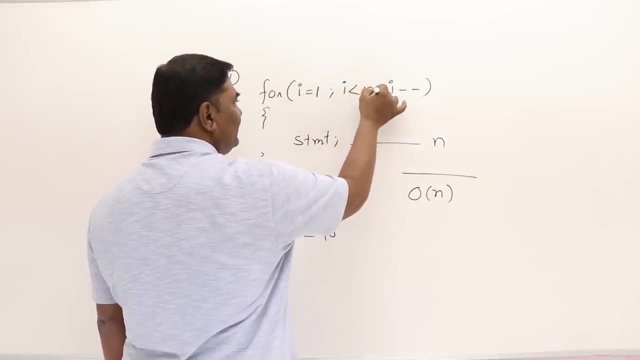 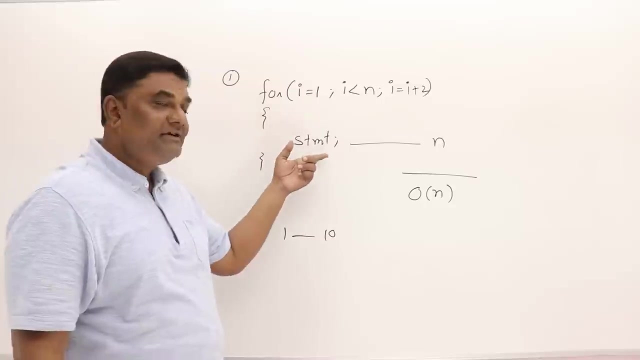 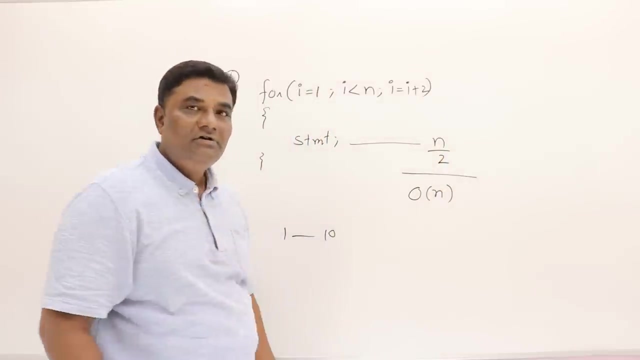 number of steps. So that's how n to 0 it is. So it is also order of n. If this is starting from 1 and condition is less than n and i is being incremented by 2.. So this statement will not repeat for n times, but half of the n times: n by 2.. If it is n by 2, also if I say function, 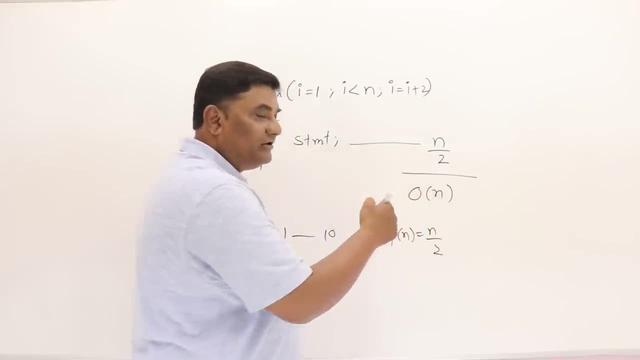 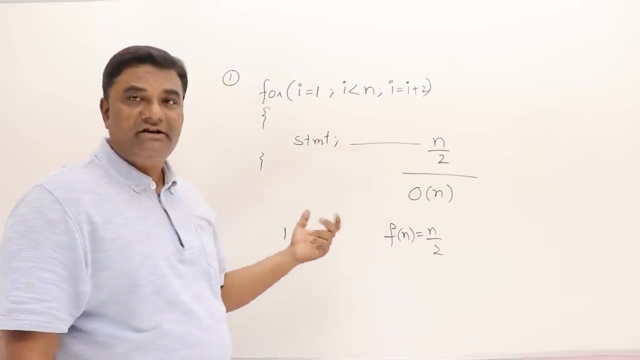 is n by 2, what is the degree of polynomial N? only, So it's order of n again. So you can. So in this case also it's order of n, Even if it is incrementing by 20, then this is: 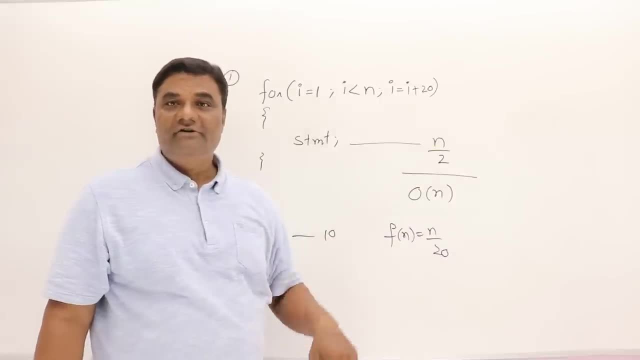 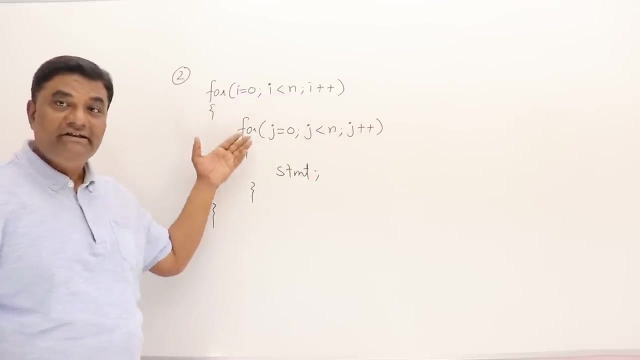 20. Degree of a polynomial is n, So this is also order of n, So n. by anything, whatever the number of times it is incrementing, the time will be same only Next. we are already familiar with this one. These are two loops, nested loop one inside another, And this: 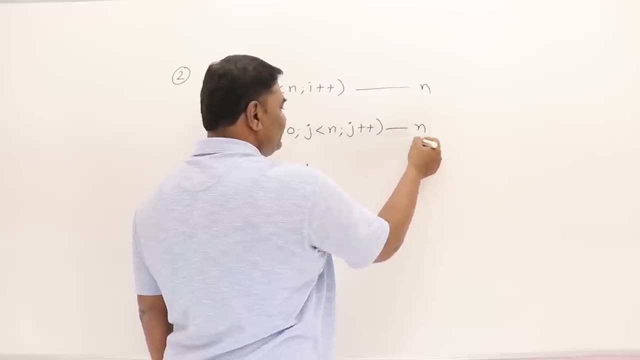 we know this will execute for n times, So this is also n times, and this is also n times. Actually, it is n plus 1.. But what about this one? Again, this will repeat for n plus 1 times, and this will repeat for n times. And this is order of n square. The next is again. 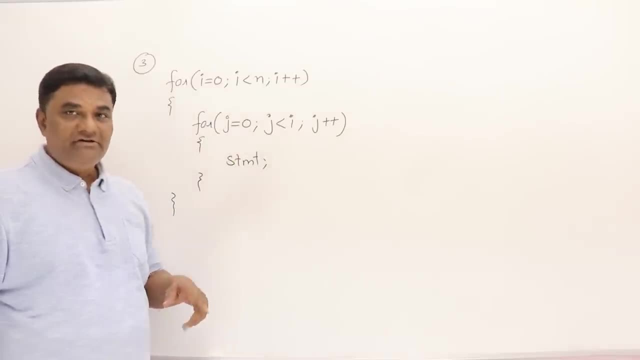 nested for loop. This looks similar to the previous one, but not See. i takes value of 0 and less than n, But j takes value j less than i. So here is the difference. So let us analyze this by tracing. 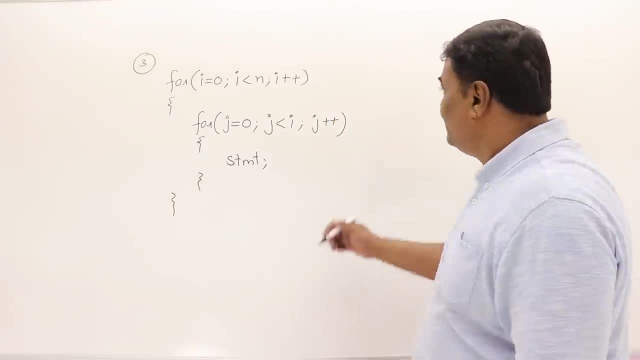 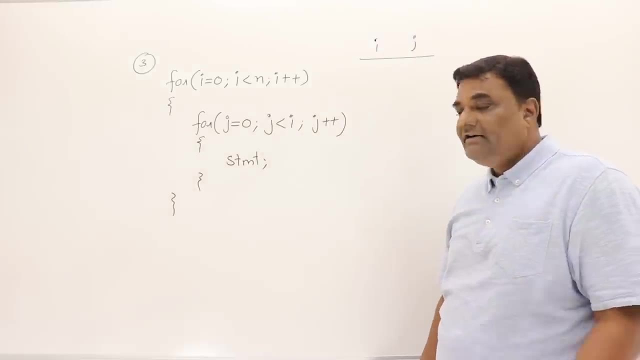 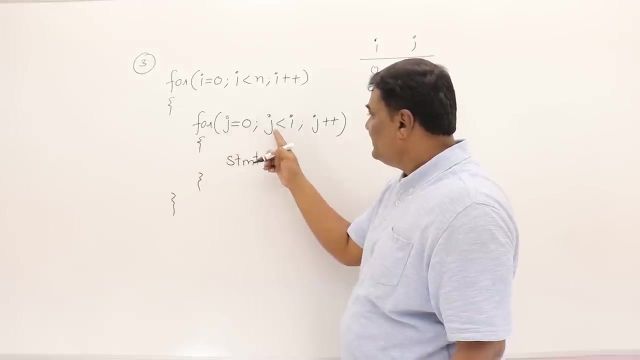 this one and find out how much time it is taking. So for this I will take i value and j value and trace them. Let us start Initially. i is 0. When i is 0, j starts from 0 and 0 less than 0. No, it will not execute for any number of times. So here I am going. 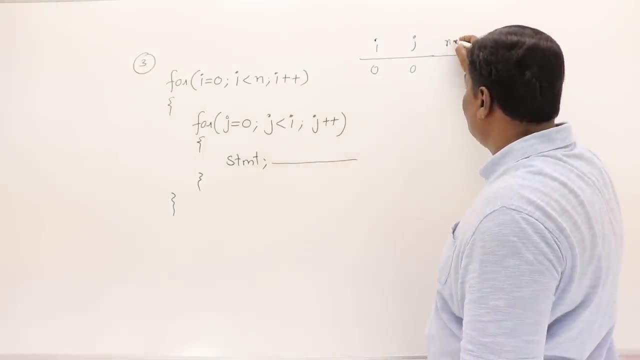 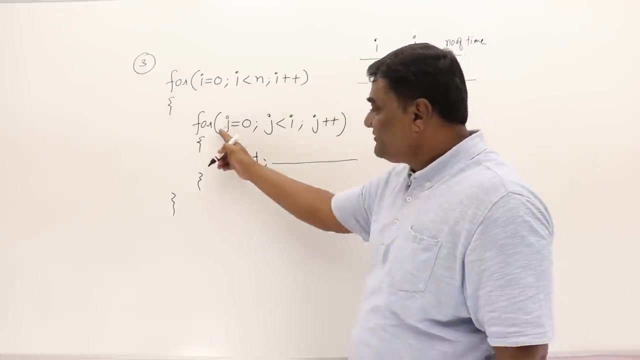 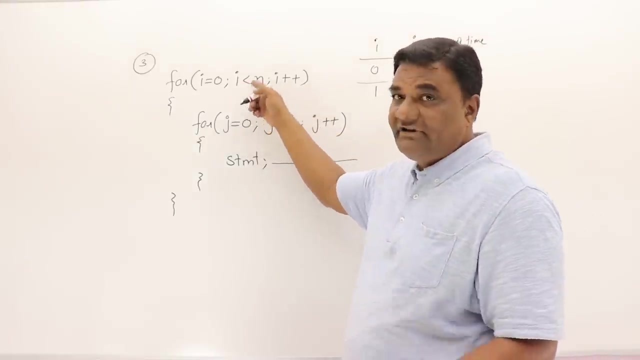 to find out how many times this statement is executed. So number of times So it will not execute at all. So 0 times. Then this loop ends Again. i plus plus i becomes 1.. i is less than n. suppose It is entered inside. Then again this loop: 0.. 0 is less than. 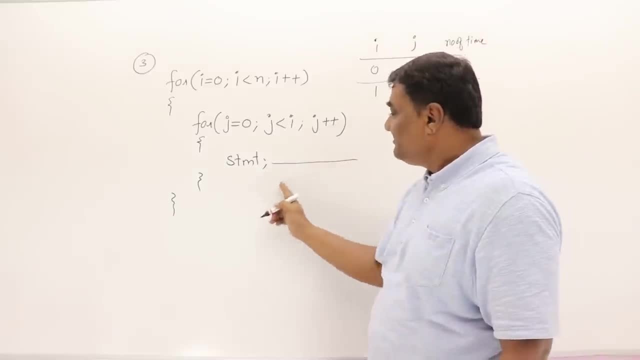 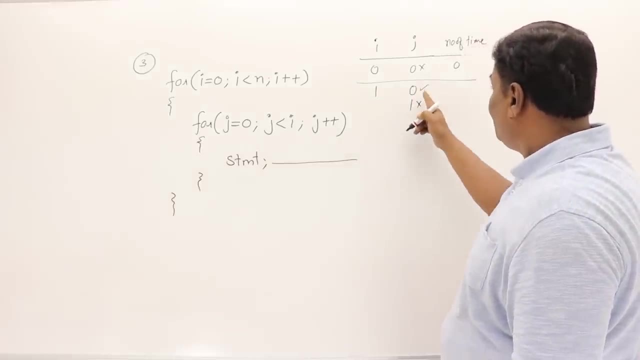 i Yes for 0, it will execute. Then j plus plus j is 1.. 1 is not less than i, So j is 1.. So for 1, it will not execute. So how many times it has executed? One time Then. 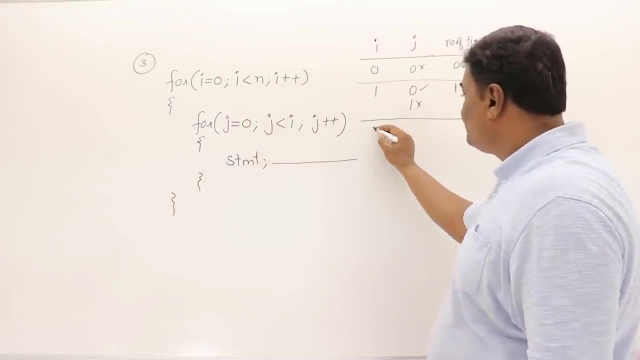 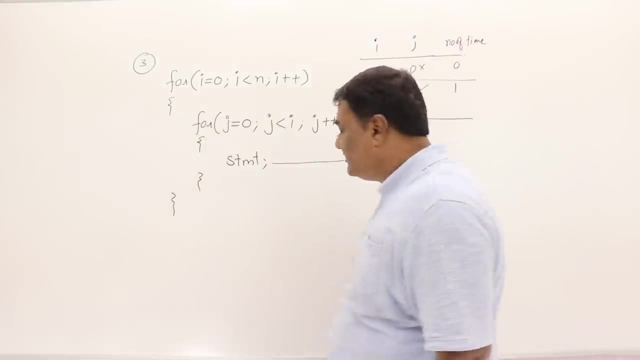 goes up again, i plus plus, i becomes 2.. Then j will execute for 0,, 1.. And when it becomes 2, it will stop. So this will repeat for 2 times, And when i is a 3,, j will take 0,. 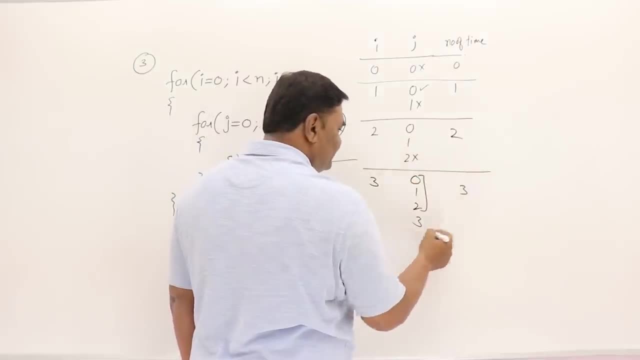 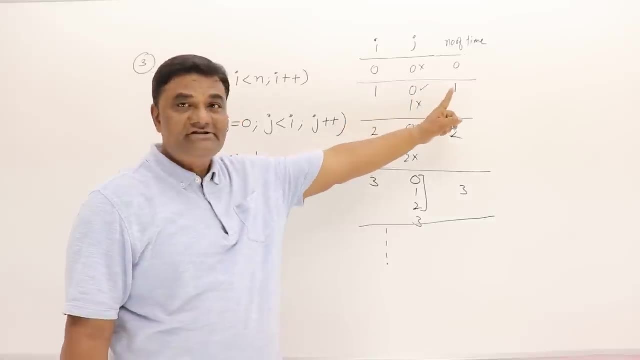 1,, 2, and 3.. So this will repeat for 3 times And this process continues. See when i was 0, it was never executed. When i was 1, it was executed for 1 time. This is statement. i was 2, it was executed for 2 times, 3,, 3 times. So 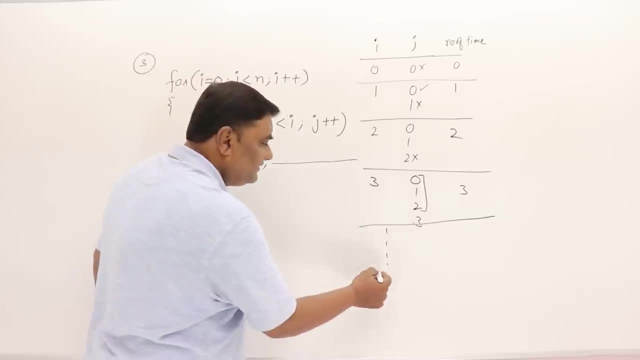 on, So on, Up to what n? So total when it is n right. how many times this will execute? n times When i was 3, so 3 times. So if it is reaching till n, actually it is less. 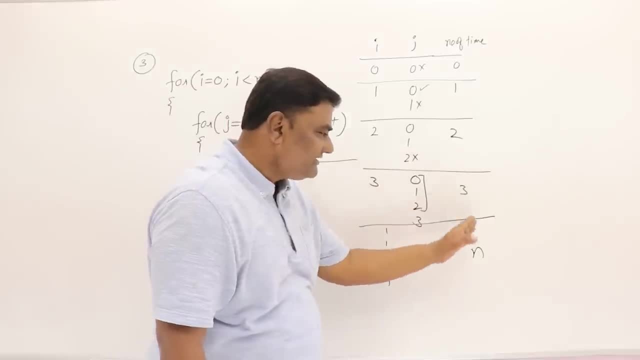 than n, But let us say n. It is reaching till n, So it will execute for 10 times. So total how many times it is executed. This one Right? So I am assuming that it is going till n, Though it is not. 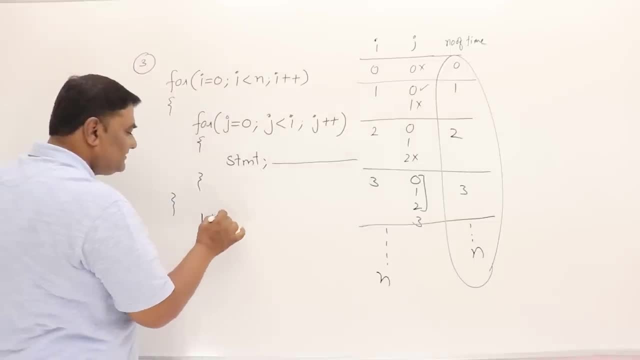 till n. it is less than n. How much that is 1 plus 2 plus 3 plus goes on to n. This is nothing but n into n plus 1 by 2.. What is the degree of this? 1. f of n is n square plus 1 by 2 degrees square. So order of n square. So the time. 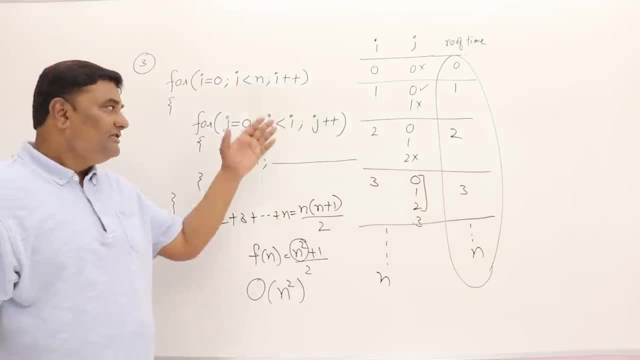 complexity is order of n? square, Though this is not similar to the previous one, but if you analyze, the answer is coming to n? square only. The degree of a polynomial is n square only. Next code is here: p is initialized to 0 and. 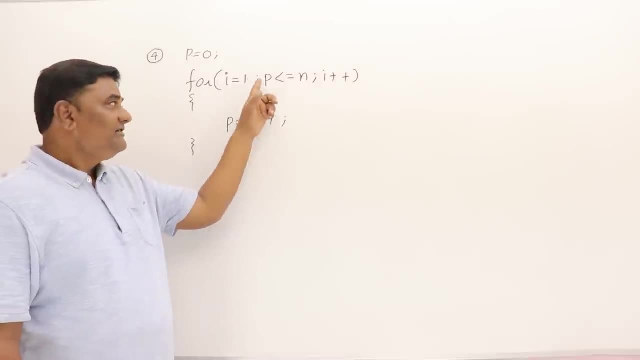 loop. This is not going to execute for n times. See this p: p is less than equal to n. It is not i less than equal to n, So the condition is different. Then what is p? p is initially 0, and every time i is added to p, So now we do not know how many times it. 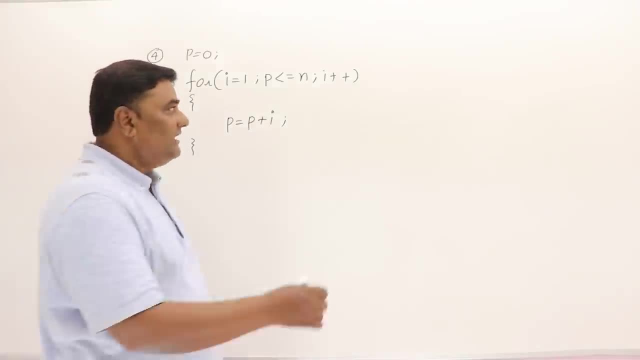 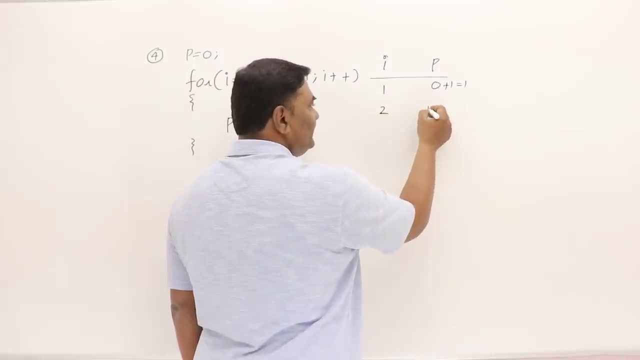 is going to execute. Let us analyze. I will take i value and p value. Initially this is 0 and this is 1.. So what happens first time This 1 is added and it becomes 1.. The next time it will be 2.. So it will be 1 plus 2.. 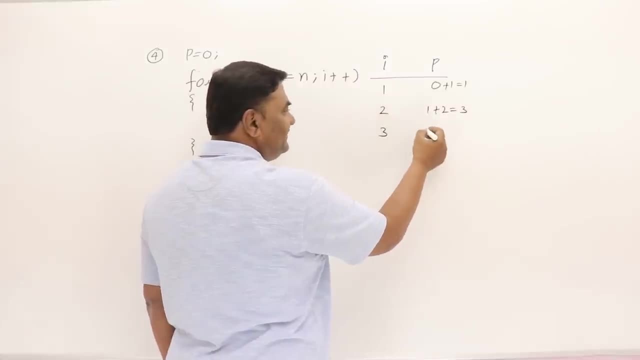 So it will be 3.. Then next time i will be 3, and this will be 1 plus 2 plus 3.. Then i will be 4.. It will be 1 plus 2 plus 3 plus 4. It goes on How many times it is going. 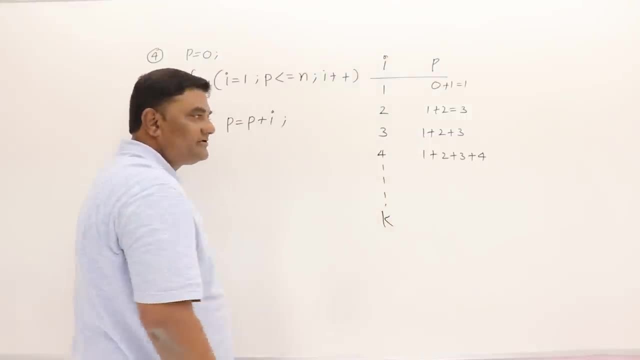 to execute. It is going to execute for k times. So what this will be? This is going to be 1 plus 2 plus 3 plus 4, plus goes on to k times. Why i wrote k here? It is not reaching It. 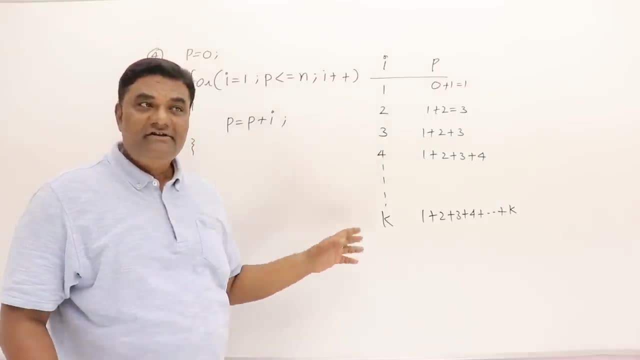 is not repeating for n times. Definitely it is repeating for some number of times that we do not know. We are sure that it will not execute for n times. Then how many times? Because the condition is different. So i said, let it be k and let us find out that. 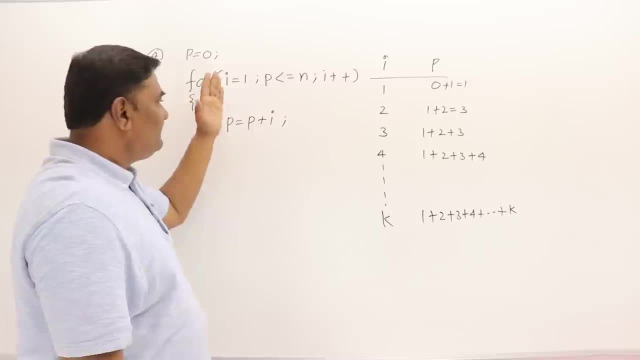 k. So if it is repeating for k times, then what is the condition? It is going to be 1 plus 2 plus 3 plus 4. plus goes on to k times. So what is the condition? We assume that p has become greater than n. So when p became 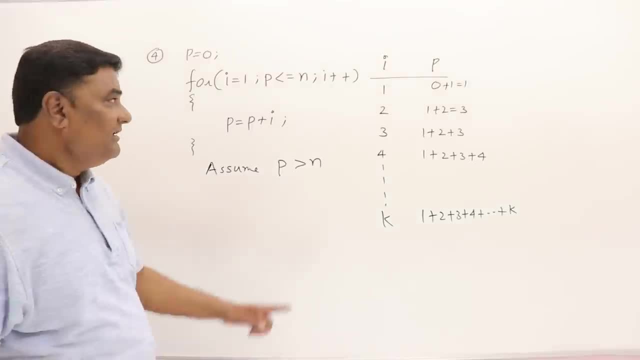 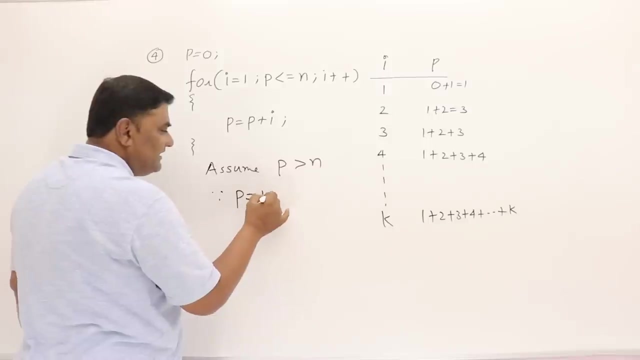 greater than n, it is stopping. We assume this. As long as p is less than or equal to n, it is repeating. So when p becomes greater than n, it is stopping Right. Since p is what Cp C, It is k into k plus 1 by 2.. p is k into k plus 1 by 2.. So when p becomes 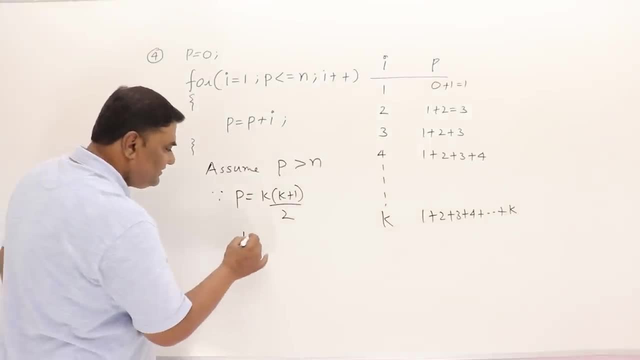 greater than n. it is repeating. So what is the condition? k into k plus 1 by 2 is greater than n. So when it will stop? When k into k plus 1 by 2 has became greater than n, it will stop. So what is k? Roughly, we assume it as k square. So what is k? k is: 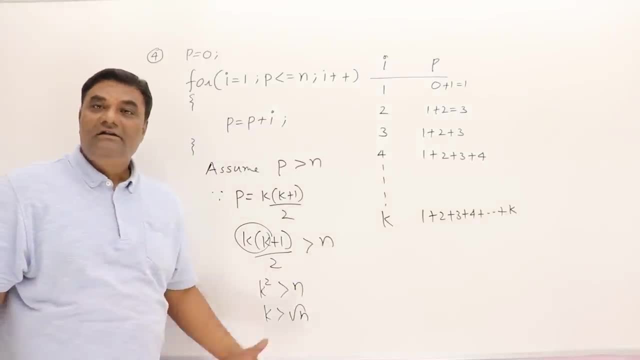 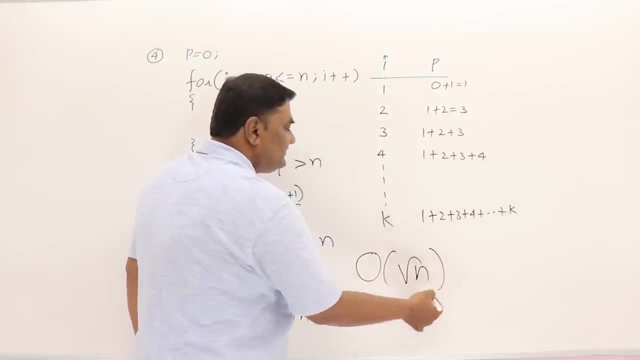 root n? k is root n. So what is k? k is root n. So what is k? k is root n. So what is k? k is root n. So this loop will execute for order of root n times. Let me show you. 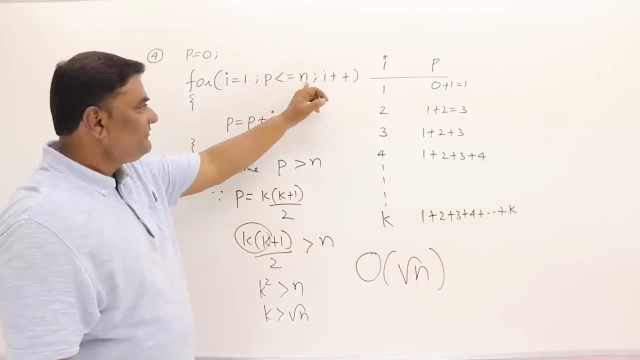 quickly, I assign: 1. p is less than or equal to n, I plus this- This is not i- less than or equal to n, So we do not know how many times it is repeating. i is here, p is here. 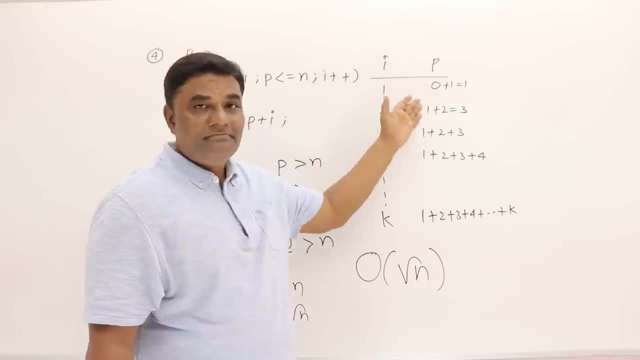 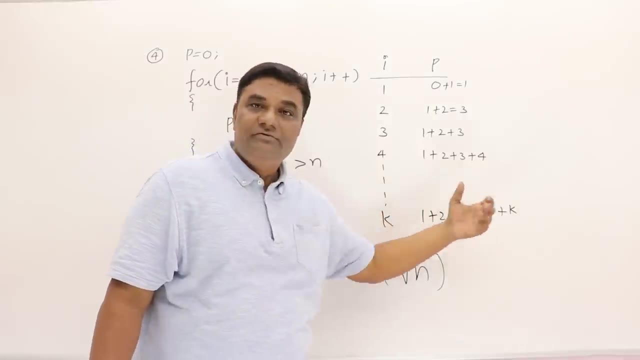 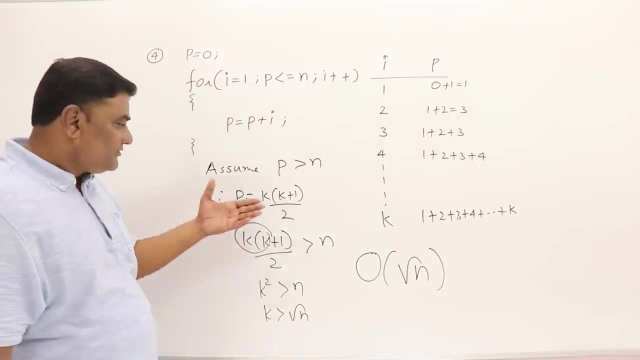 So i values are incrementing, and every time i is added to p, So we do not know how many times. So let us say k times, And this will be 1 plus 2 plus 2 to k, Right, So that k is.